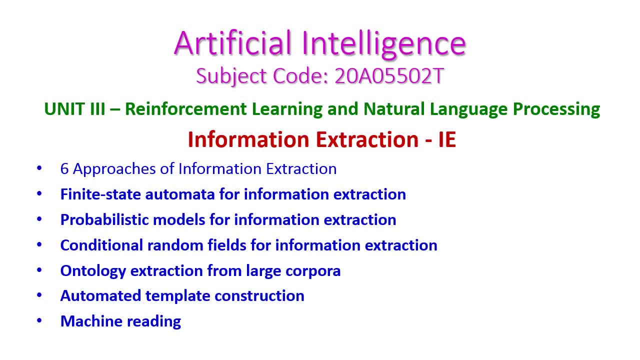 In this artificial intelligence class we will see another important topic from third unit, that is, information extraction. that will come under NLP. So in this information extraction class we will see what is information extraction and the six different approaches of information extraction, like the finite state, automata and probabilistic model, conditional random fields and ontology extraction and automated template construction and machine reading. 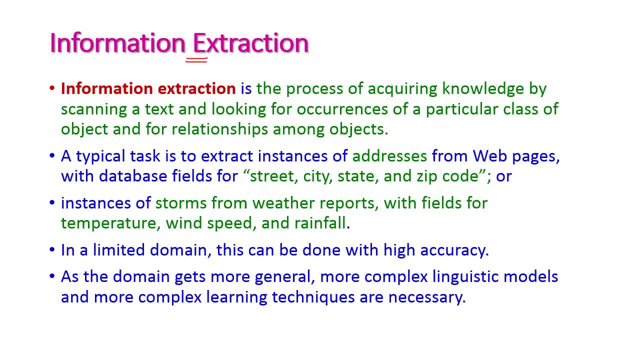 What is information extraction? So it is a process of acquiring knowledge by scanning text and looking for occurrence of particular class of objects and the relationship among object. so this is called as information extraction. that is, by scanning a text we try to get some knowledge from the test. okay, for example, suppose we want 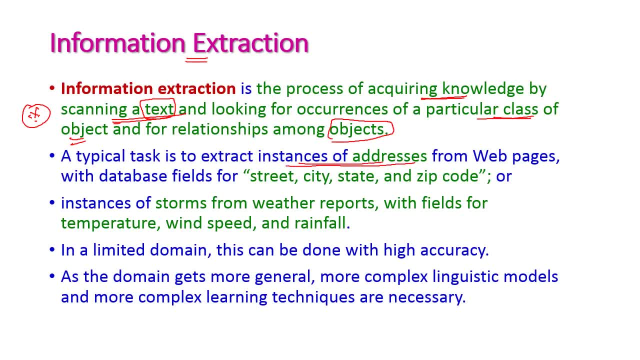 to extract instance of addresses from web page. okay, for getting the address. the database field require are the street, city, state and zip code. so these are the field we required to get address right. when come to second example- suppose the storm of weather report- we want the storm of. 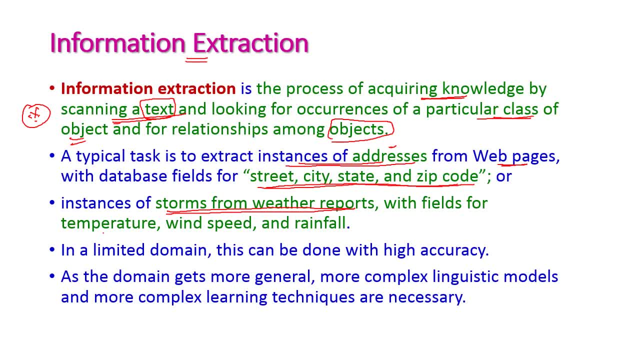 weather report. for this the required field are the temperature, wind speed and rainfall, right, so by this way, from the given information, we need to get some knowledge. okay, so this is called as information extraction. if the domain is very limited, then the accuracy will be very high, okay. 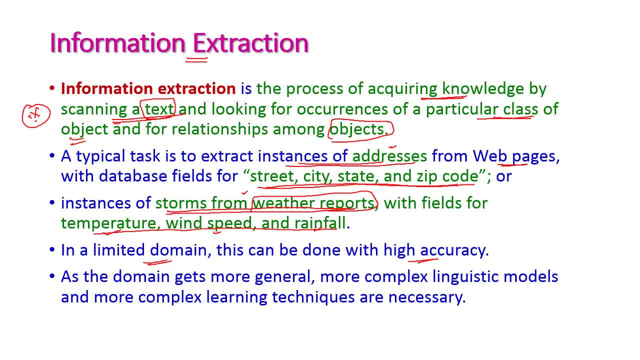 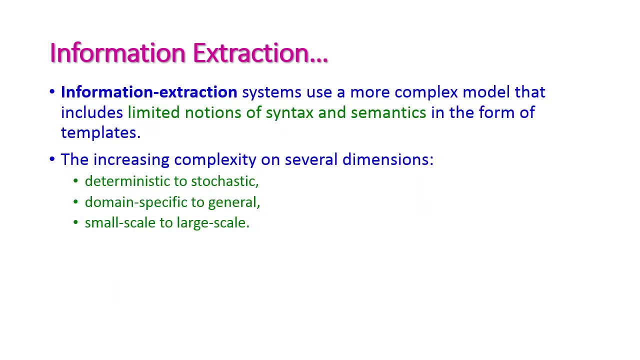 knowledge accuracy will be very high. but if the domain is more general domain, okay, then we required some more complicated learning technique to get the knowledge right. this system uses more complex models, which includes limited notation of syntax and semantics. okay, in the form of templates. why? because the complexity will get increased day by day. that is deterministic to stochastic domain. 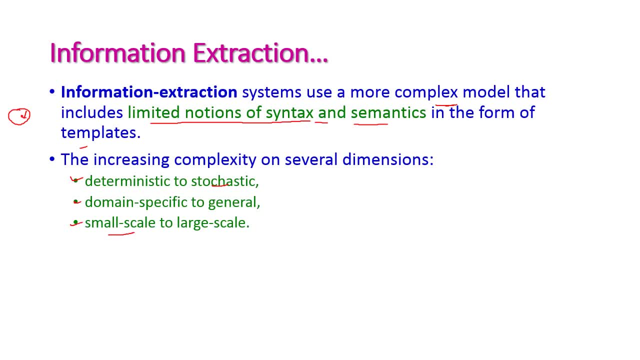 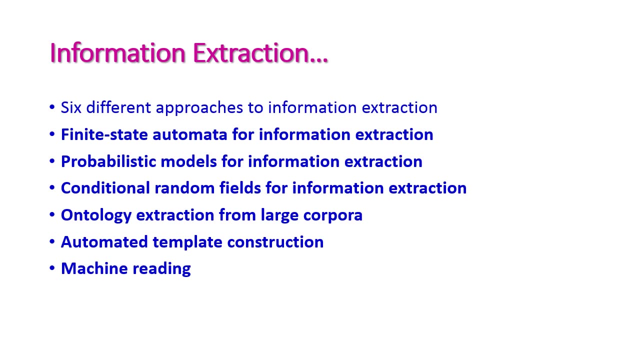 specific to general, and small scale to large scales. that is, the domain got increased day by day. hence the system uses more complex model with limited notation of syntax and semantics right. the six different approaches are used to get the knowledge right, so this is called as information extraction. 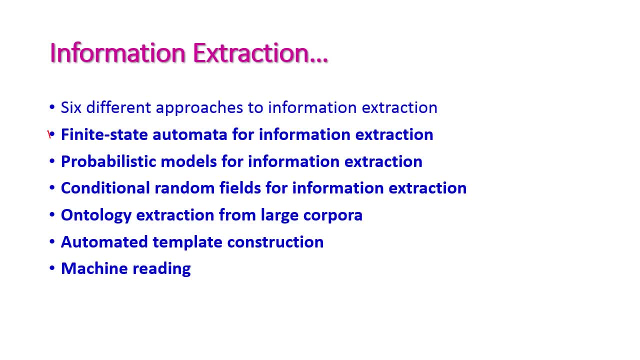 in information extraction. first one is final state automata for information extraction and second, one probabilistic model for information extraction. and third, one conditional random field for information extraction. and fourth one ontology extraction from large corpora. and fifth one automated template construction. and sixth one is machine reading. let us say all those things one by one. final state: 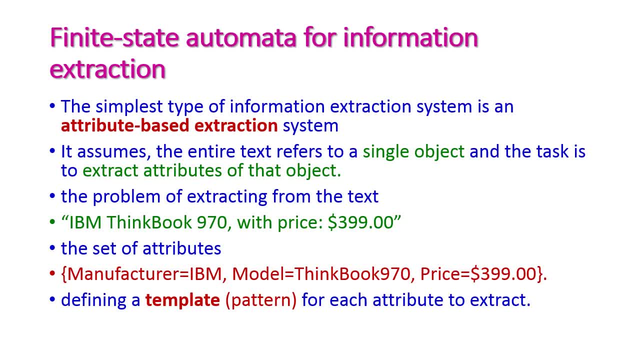 automata for information extraction xf. uh, let us try both to i as record: ah, ah, 970, with price: 399 dollar. okay, this is the the set of attributes. from this we try to extract the attribute. what are the attribute? ibm means manufacturer, the model is think book 970 and 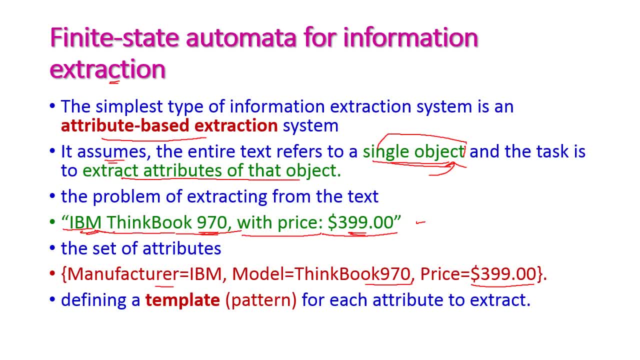 price is 399 dollar. okay, so these are the attributes. so here we have to define a template for each attribute to extract. okay, for each attribute we have to define a template so we can use this template for extracting any like the objects. okay, any similar object, we can use the same. 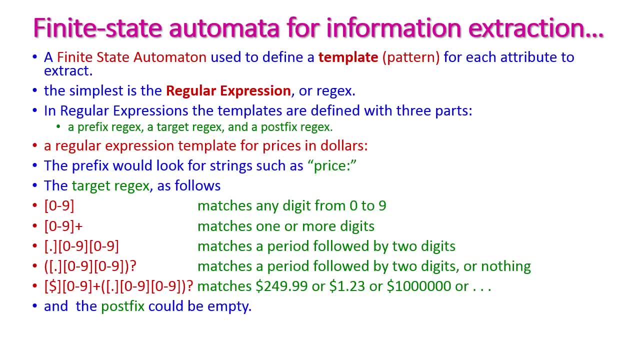 attribute, the finite state automation, which is used to define the template for each attribute to be extracted. okay, and from this finite state automata, the regular expression is the simplest one and it is having three parts for defining the attribute. first one is prefix, target and post fix. okay, let us see one. 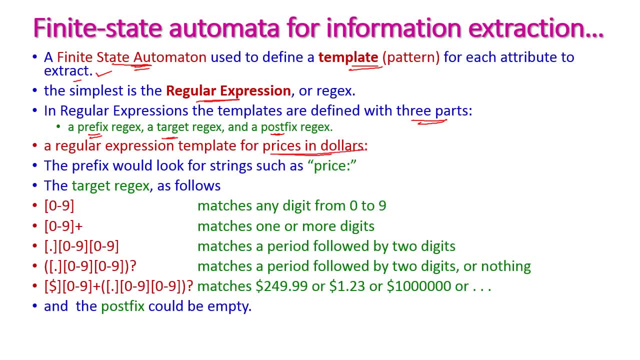 example for defining the price in dollar by using regular expression. okay, here the prefix is price, price is prefix and the target digits. so here we have to display the numeric value. if it is a single digit, we can give likewise. so the numbers 0 to 9 will be printed here if we 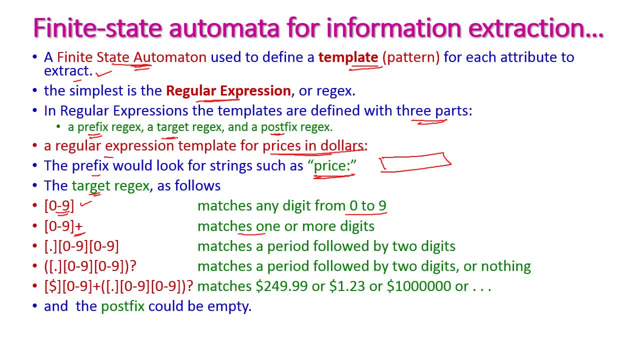 include plus sign followed by digit means one or more digit will be displayed here. okay, suppose point followed by two digit means so the period followed by two digit and the question mark means if there is a digit, that will display otherwise nothing. okay, so finally, this is our. 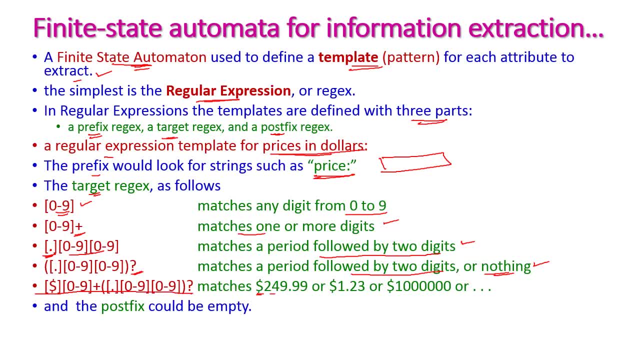 format: okay: dollar followed by one or more digit and point followed by two digit. okay, if two digits are there, that will display. if there is no digit, that won't display. for that purpose we have used this question mark. okay, and post fix is nothing, that will be empty, okay, so this is how we have to give. 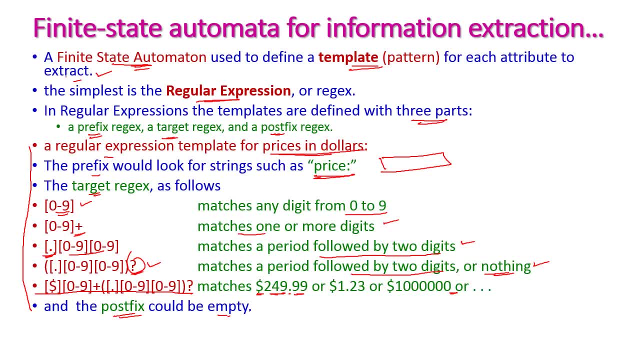 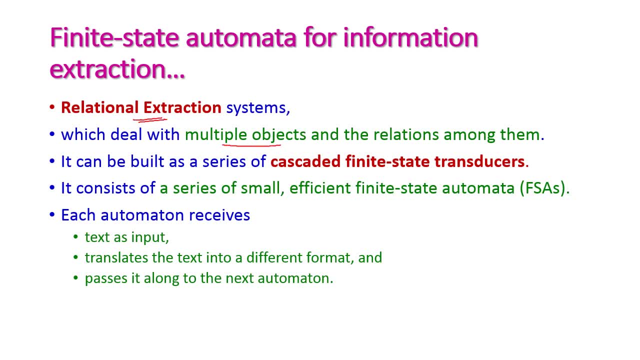 format for all the attributes: relational extraction: a relational extraction system which deals with multiple objects and relations among them, that is, from the given input, plain text, it identifies the object and it will find the relation between the objects also right, and it can be built with a series of 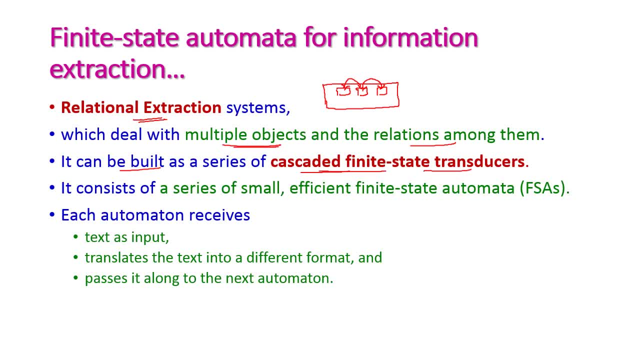 cascaded finite state transAULT, PER Да, who consists of a series of small, efficient FSA, that is, finite state automata. Here, each automation receives a text as input and the input data will be translated into different format, and this different format will be passed to next. 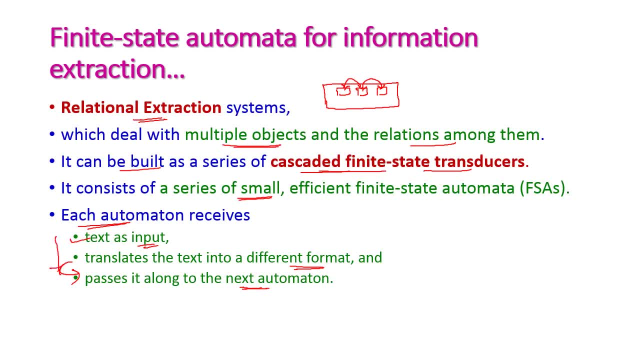 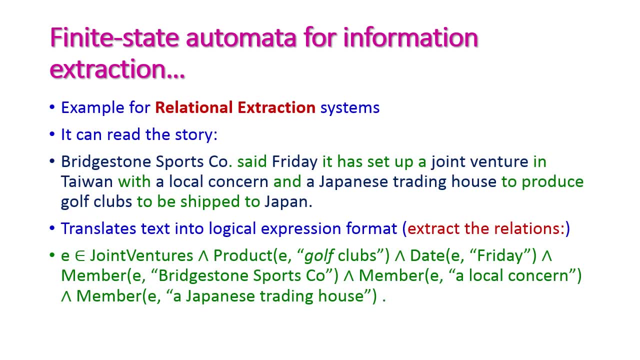 automation. okay, So this is called as cascaded finite state transducers. Let us see one example for this relational extraction system. First one is: input the given story. okay, The text will be given to our relational extraction system, okay. 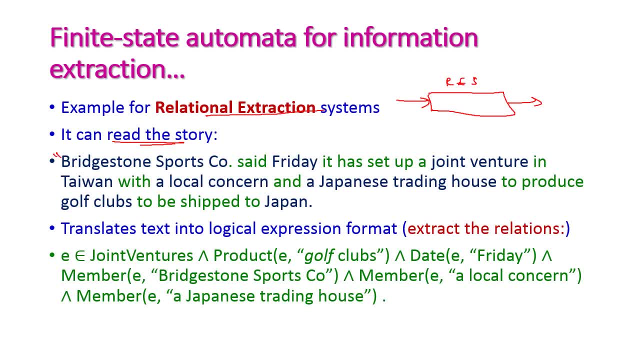 And the plain text. this is our plain text and this will be given to our system as input. So here the objects are highlighted in different color. okay, So after finding the object, we have to create the or identify the relationship among the object. 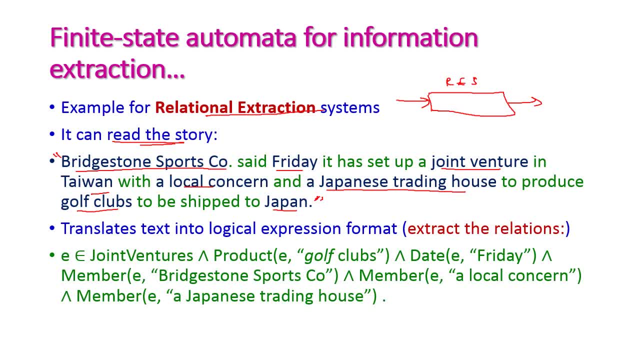 By using given verb. okay, So after identifying all those things, that is, after extracting all those things, the text will be translated into logical expression format. okay, The given text will be changed, that is, converted into logical expression format, And this logical 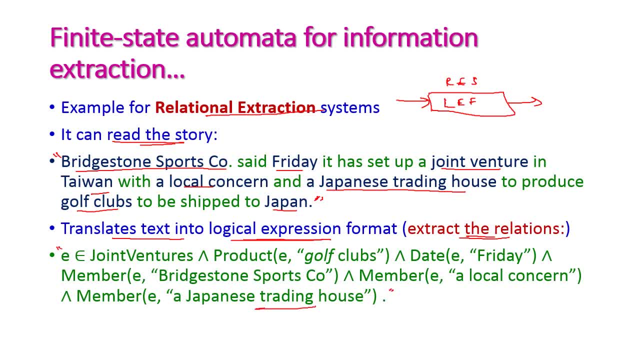 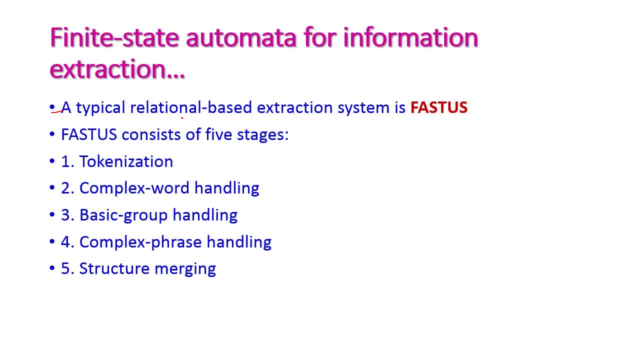 expression format will be given to the next step, next iteration. A typical relational based extraction system is fastness. This fastness consists of five stages. First one is tokenization, complex word handling, basic group handling, complex phrase handling and structure merging. okay, So we will see all these five stages one by one. 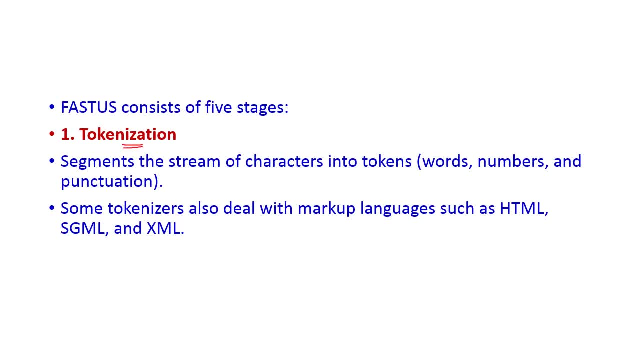 The first one is tokenization. Tokenization means segments the stream of character into tokens, that is, from the given sentence of character that will be divided into words, numbers and punctilations. okay, So a small word is called as token and this tokenization can also implemented in html, html and xml. and second one is complex word handling. 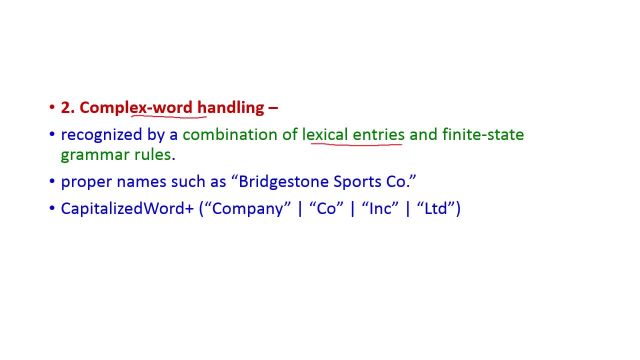 Complex word means more than one. logical entities will be there and this will be identified by using finite state grammar rules. Okay, See, this is a single name and this may be a complex word. okay, That is more than one. lexical entities are there. 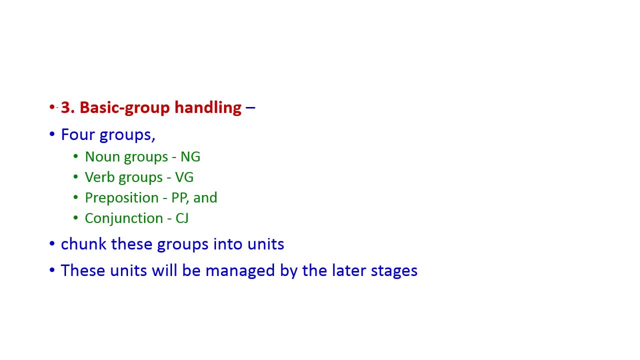 The third one is basic group handling. When come to basic groups, there are four groups are there. First one is noun group, NG, verb group VG, and these two are most important group basic groups. The third one is proposition PP and fourth one is conjunction CJ. So these four are the basic groups. 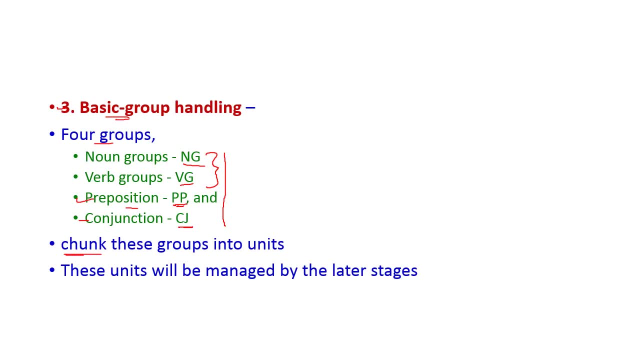 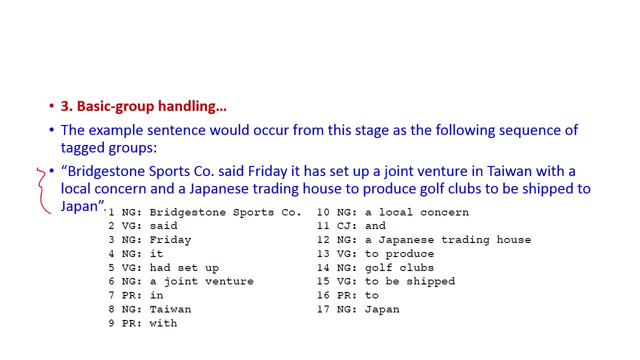 Here the given text will be chunked into these groups, into unit okay, And the units will be merged into here. this is the given input string and this input string will be divided into the sequence of okay. So, as per our example, we are having 17 tagged group. Here we can see all the groups, noun group, verb, group proposition and the conjunction okay. 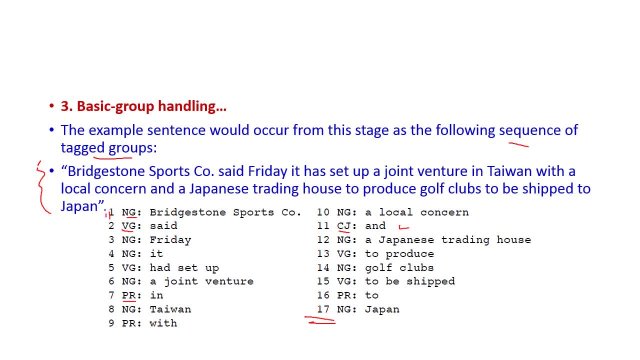 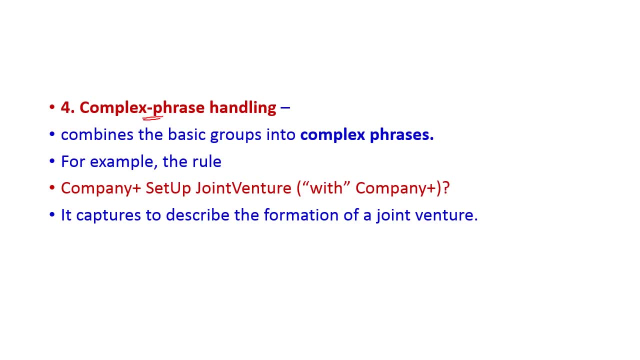 According to this, the given string will be converted into different subgroups. The fourth stage is complex phrase handling. That is, the basic groups will be combined to form these complex phrases. For example, the given rule: Company plus setup joint venture of with company plus, and followed by question mark okay, 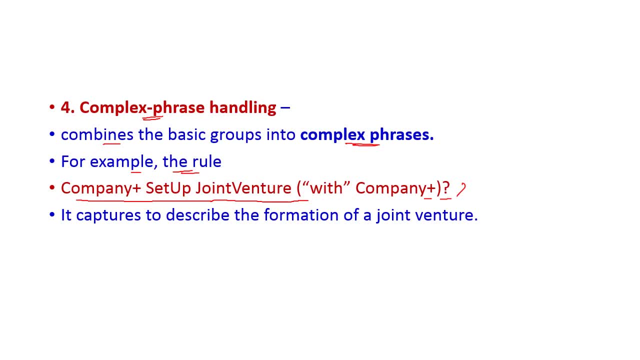 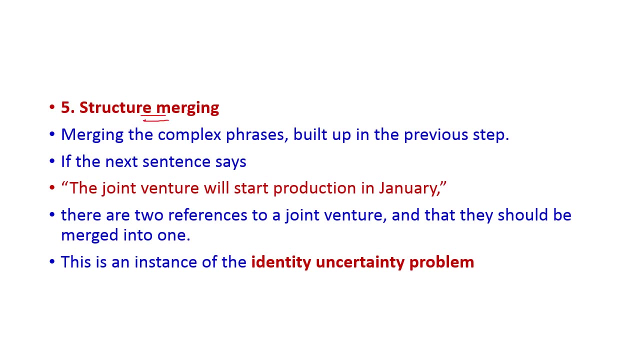 So it captures how to describe the formation of joint venture. So joint venture. here the joint venture will be displayed, in which format? that will be described here. The last stage is structure merging. This will come from the previous step, that is, merging the complex phrases. 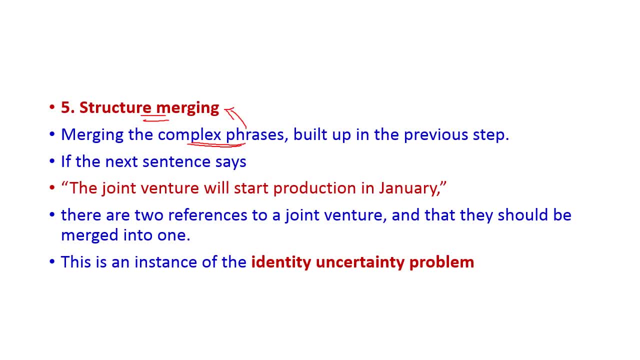 Okay, Merging the complex phrases is called as structure merging. So the given sentence: the joint venture will start production in January. okay, Here there are two reference to this joint venture. okay, And they should be merged into one. okay. 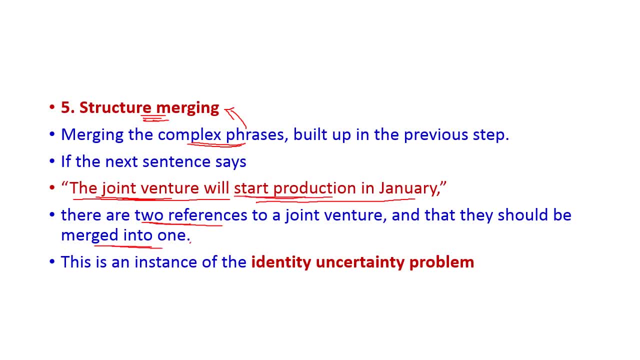 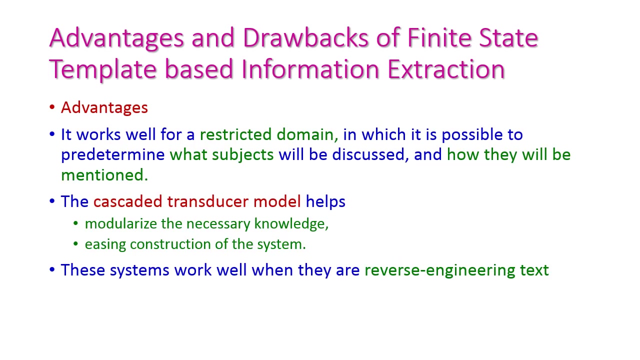 So this will start production is one reference. In January, when it will start production In January, this is another one. So everything should be merged into one single sentences And this is an instance of identity uncertainty problem. The advantages and drawbacks of finite state template based information extraction. 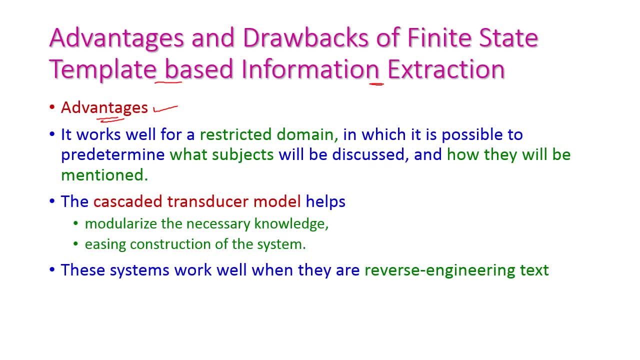 First let us see the advantages. These systems will be very much suitable for the restricted domains. If the domain is very specific, then the system will work well. In this domain, it is possible to pre-determine what subject will be discussed and how they will be mentioned. 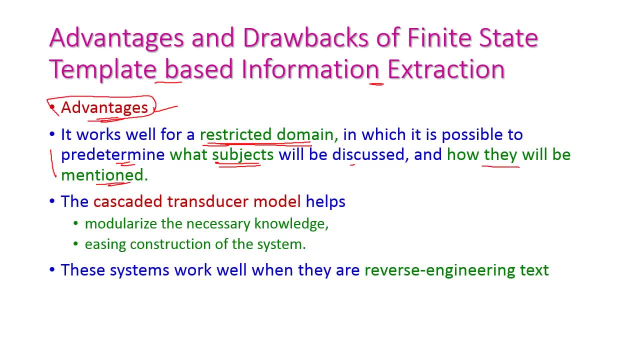 If it is possible, then the system will work very well, And when come to the cascaded transducer model, it is very much helpful for modularizing necessary knowledge and easing construction of systems. okay, If the system is very simple, then we can easily use this. 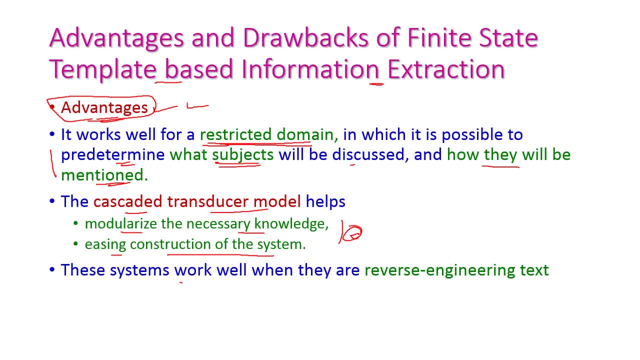 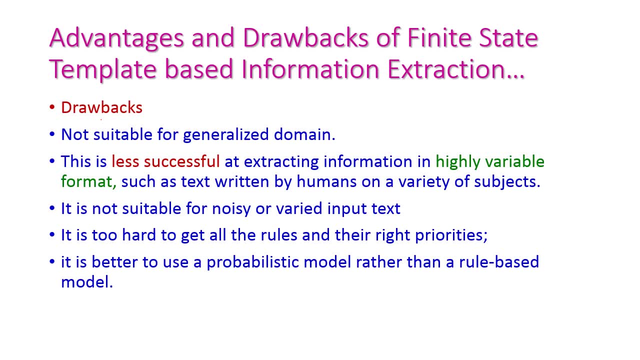 And this system will be very much suitable for reverse engineering text. And next let us see the drawbacks. And this system is not suitable for generalized domain. If it is specific domain we can use, but when come to generalized domain, the system will not be used. 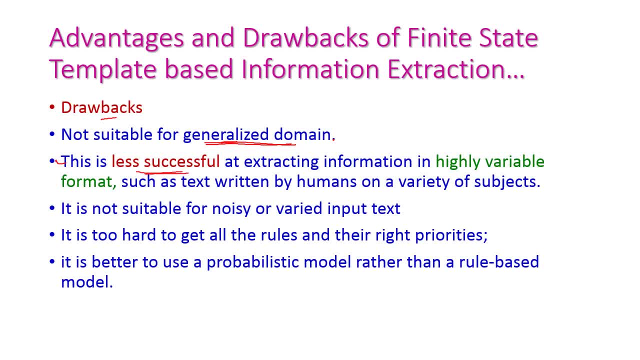 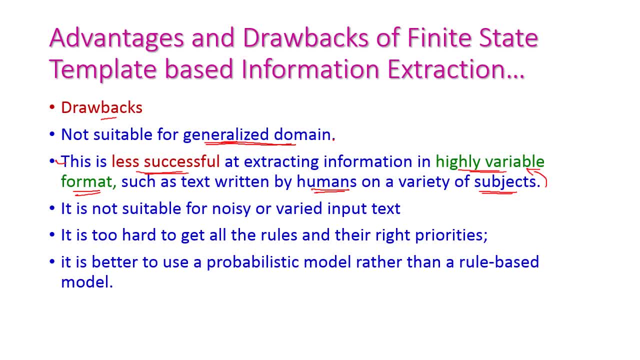 And if the format is written by human And if more number of subjects included, then this is less successful And it is not suitable for noisy text or varied input text And it is too hard to get all rules and their priorities okay right priorities. 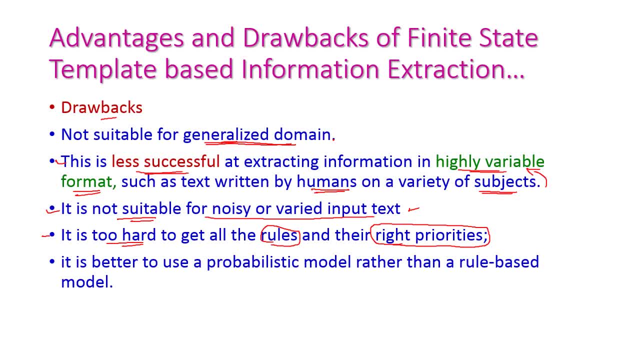 Which rule will come first, which rule will come next are defining is very hard, And in those situation we can use the probabilistic model instead of using this, And in those situation, we can use the probabilistic model instead of using this. 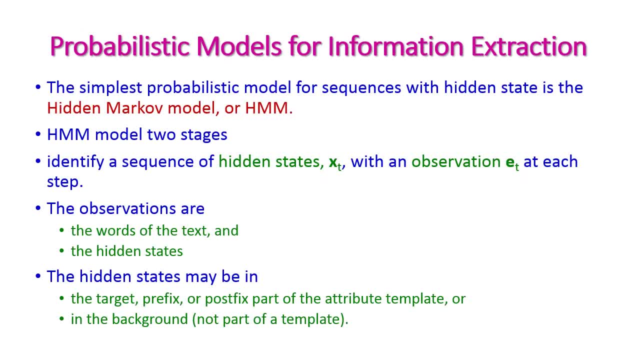 And in those situation, we can use the probabilistic model instead of using this Rule based model. The probabilistic model for information extraction. The simplest probabilistic model is hidden Markov model, which is otherwise called as HMM. In HMM, there are two stages. 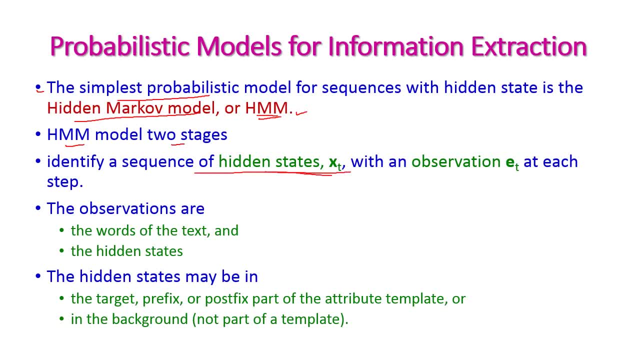 First, it will identify a sequence of hidden states, which is represented by Xt And the corresponding observation, that is Et, at each step And the observations are, That is Et, Observations are the words of text and the hidden states, So these to be observed. 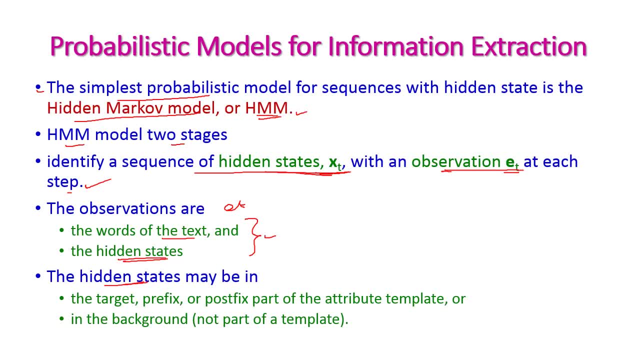 And when come to hidden state, it may be a target or prefix or postfix. part of attribute template, Okay. otherwise, in the background, that may be not part of the template. Okay, so these are the hidden states. Let us see one example for this. 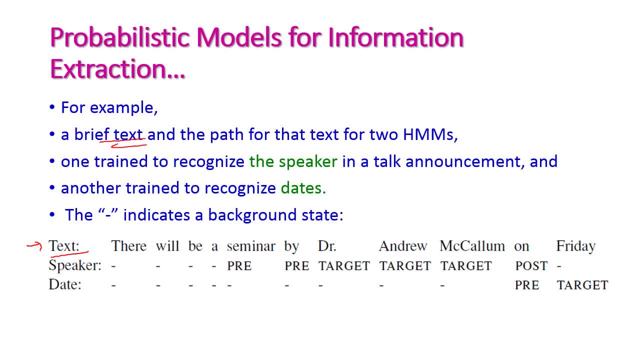 The given text. The given text. There will be a seminar by Andrew McCullum on Friday. Okay, this is the given text And the path for the text. Okay, two HMMs are trained here. First one trying to recognize the speaker. 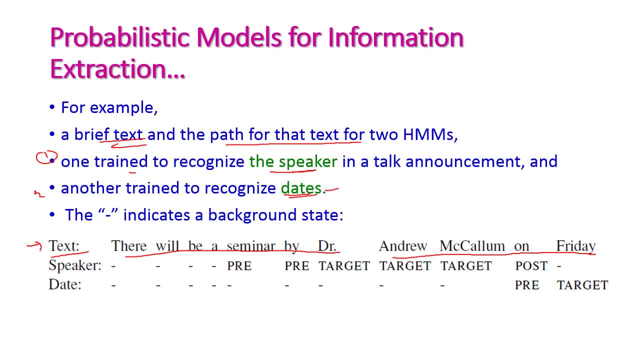 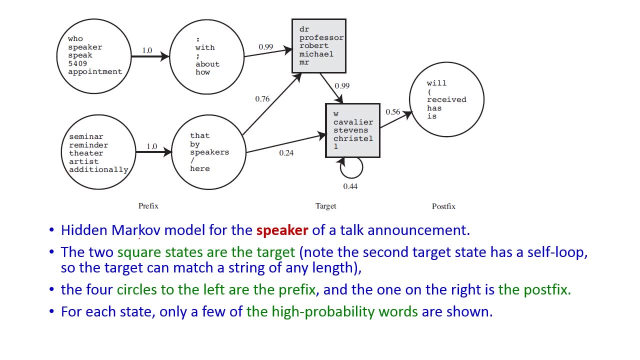 And second one trying to recognize the date. Okay, this is the second one, And the hyphen. hyphen are here. Those are used to indicate the background state. This diagram explains the hidden Markov model for speaker of talk announcement. 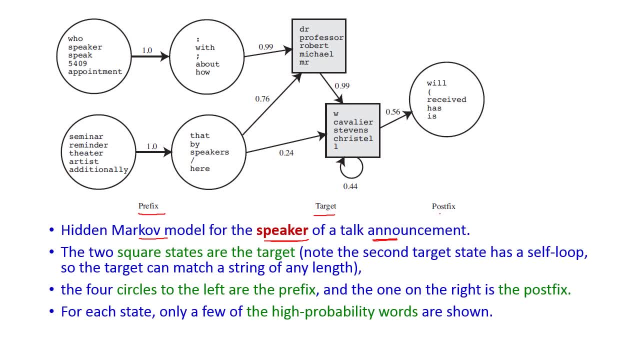 Okay, here we are having prefix, target and postfix. Target symbol is square, That is, two square states are there And these are the target. Okay, when come to the second target, there is a self loop That means the string can be. 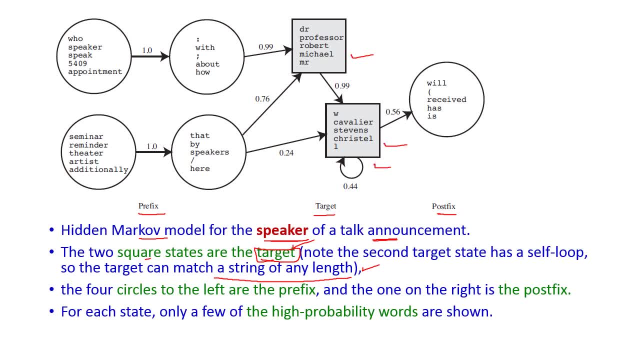 Any length Matching string can be any length That represented by self loop. And when come to prefix, four circles are there And in the postfix only one circle is there In the right hand side. Okay, and for each state only a few of high probability words are shown here in this diagram. 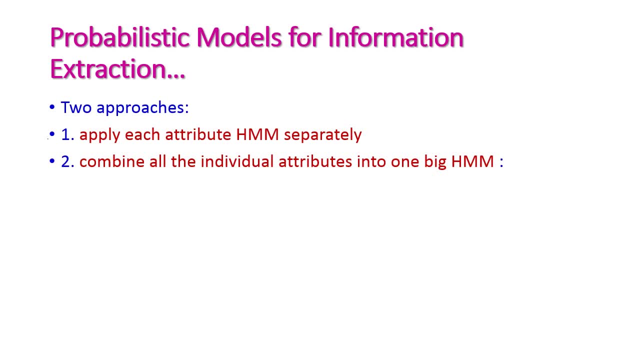 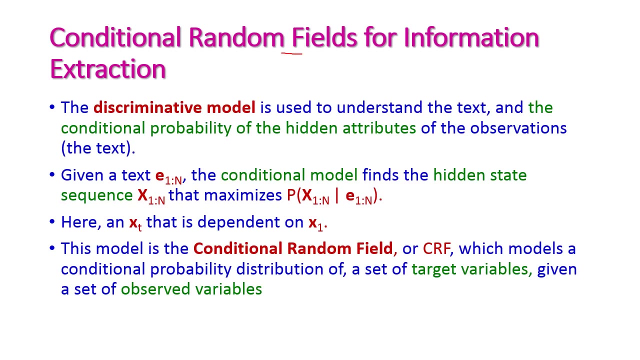 In this model there are two approaches. First one is Apply each attribute HMM separately, and second one is combine all the individual attributes into one big HMM. The conditional random fields for information extraction Here the discriminative model which is used to understand the text, as well as the conditional probability of hidden attributes of the given text. 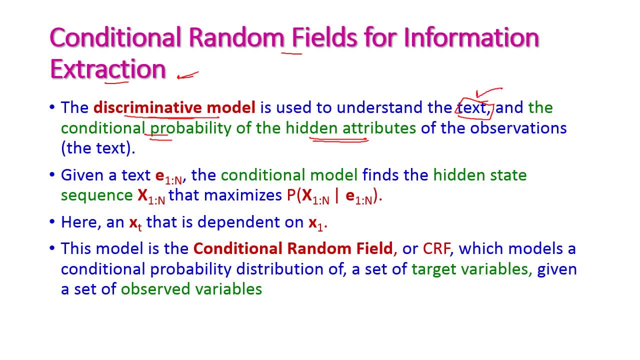 Okay, that is this model. First, understand the text as well as the hidden probability, that is, the hidden attributes of the given text. Okay, it will understand the hidden attributes of the given text. Okay, the given text will be represented as E of 1 to n. 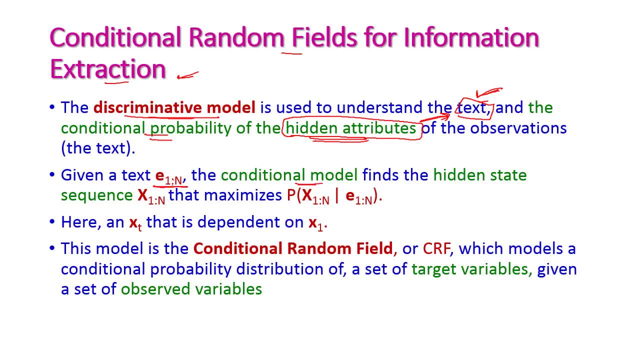 E 1 to n And the conditional model. this particular model will find the hidden state sequence, That is, capital X, 1 to n. Okay, that maximize the probability of capital X, 1 to n, such that E of 1 to n. 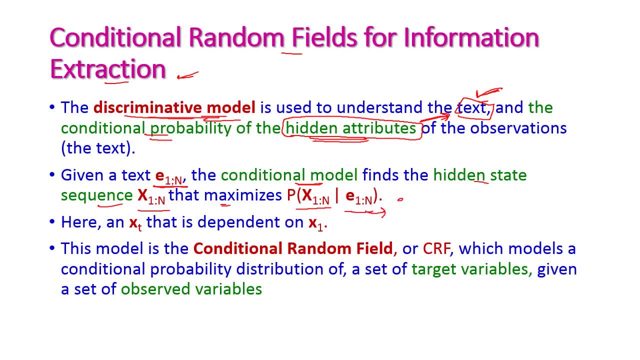 That is, E of 1 to n. is the given text Given text And from the given text the hidden states will be extracted. Okay, n number of states extracted, That is, hidden states. Hidden states will be extracted And the hidden states will be dependent to each other. 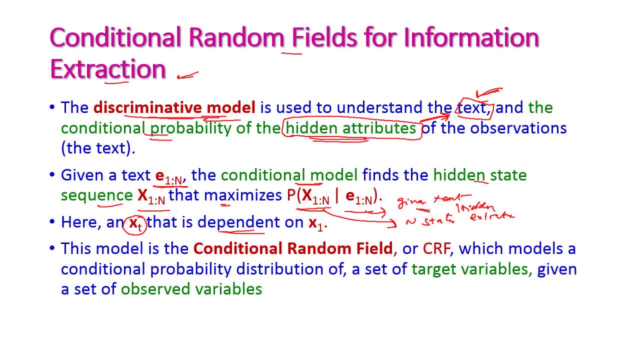 That is Xt, that is, any of the hidden state that will be dependent on X1.. Right, And the model is conditional random field- Conditional random field, which is otherwise called as CRF, which models the conditional probability distribution of. 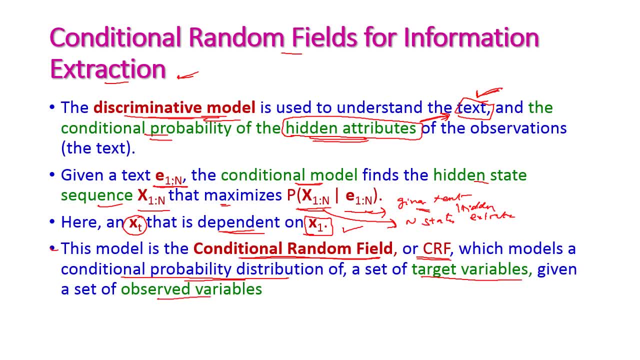 of target variables given set of observed variables: Okay, So we have to find the target variable from the observed variable. Observed variables: Okay, So the discriminative model that is used to understand this text, as well as the hidden. 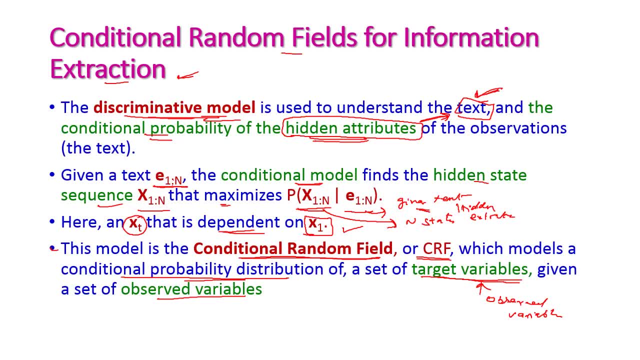 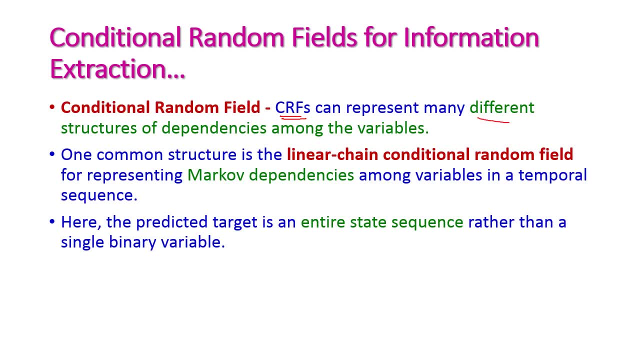 attributes of the given text. Right, Okay, Okay, here the crf that represent many different structures of dependencies among the variables. that means the hidden data are dependent to each other. in what way those data will be dependent in what structure is maintaining? here everything will be represented by this crf. okay, and from. 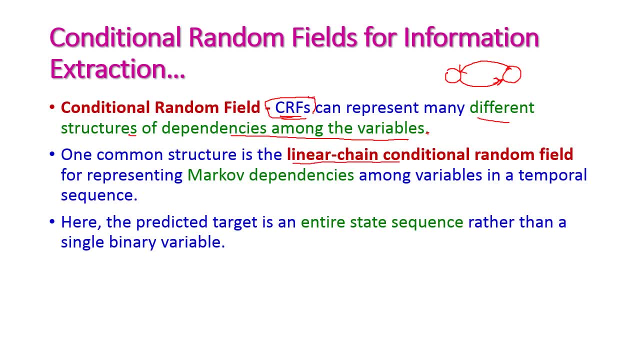 this one common structure is linear chain, conditional random field. okay, so this represent the markov dependencies among variables. okay, the markov dependencies among variables. the markov dependencies is actually available in temporal sequence, so this is one of the temporal model learning model. okay, this will represent the dependencies between the variables. 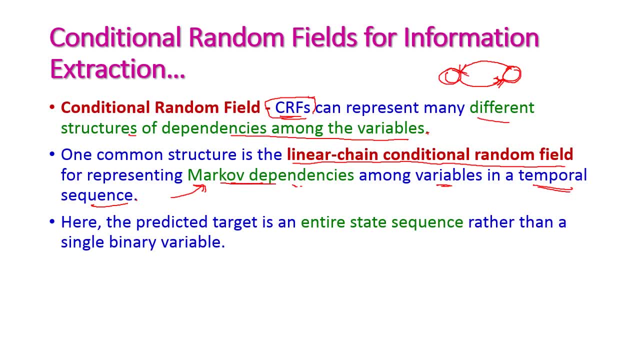 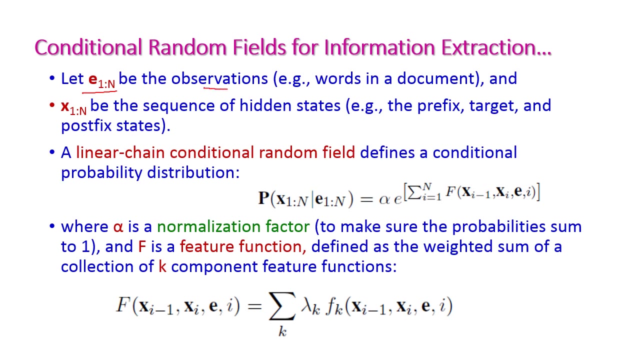 how the variables will be dependent to each other. and ah, the predicted target is an entire state sequence rather than a single binary variable. okay, so the target is the entire state sequence. so here e 1 to n is observations that may be a word document, and x 1 to n be. 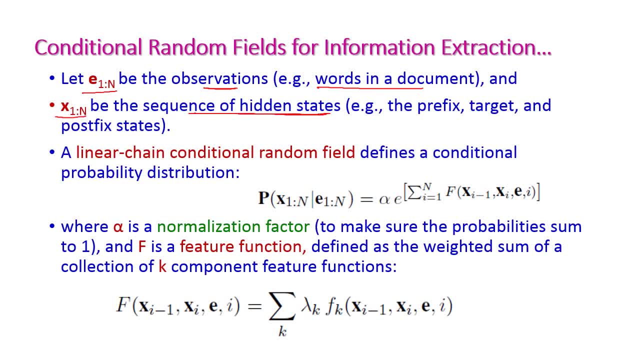 a sequence of hidden states, as we already seen. e is a given text and x 1 to n is hidden state. okay, the hidden state. for example, it may be prefix, target and post fixed states: okay, those are hidden state here. the linear chain, conditional random field which defines: 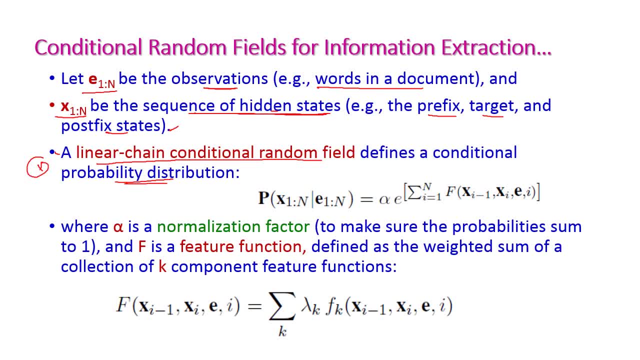 the conditional probability distribution that defines the conditional probability distribution, that is, the probability of x 1 to n, is a sequence of hidden states, as we already seen. e is a given text and x 1 to n is hidden state. okay, the hidden state. for example, it may be prefix. 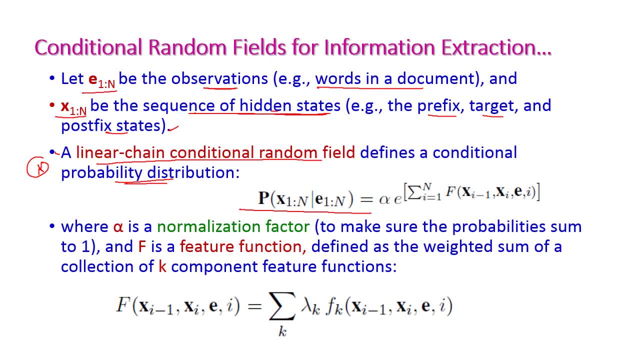 plus i equal to e, to the power h c type x 1 to n, such that e 1 to n, which is equal to alpha e. power of summation of i equal to 1 to n. capital f, f of x, i minus 1, x i e i okay. 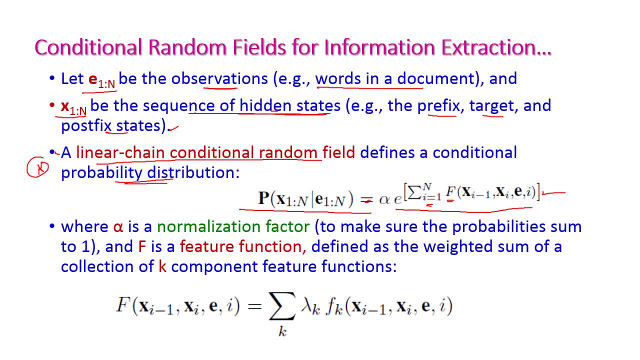 so this is the conditional probability distribution, here, alpha. so this alpha is nothing but normalization factor and f is nothing but this f. so alpha of x, 1 to n is the conditional probability distribution. here the general conditions are what it supposed to be say, by which we have: 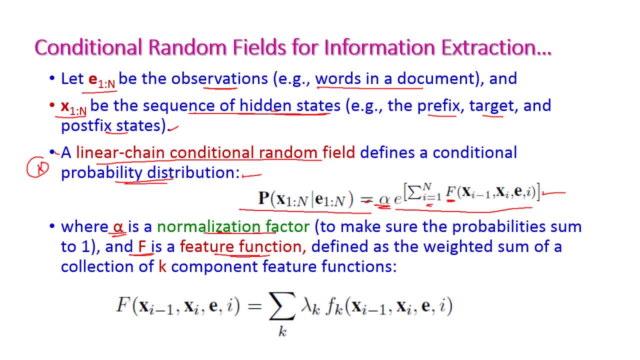 x is equal to delta x 1 to n, and x i is equal to 1 to f, once alpha. so these parameters both are equal to delta x to the power, and therefore similarly it is also agreed if we finish this, f is future function. ok, So this defines the weighted sum of the collection of k components. 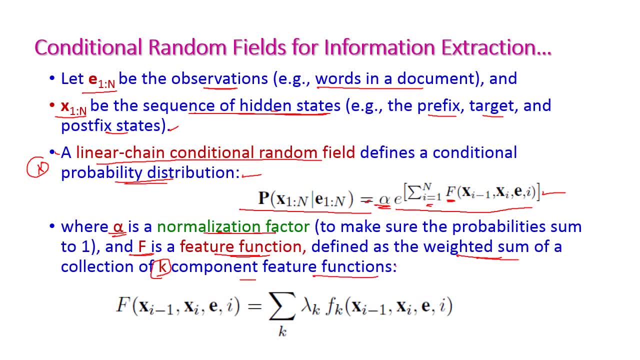 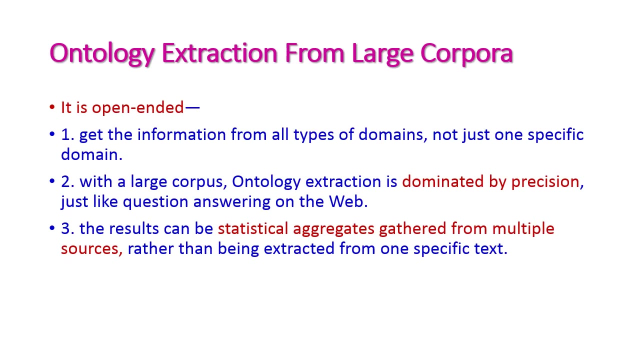 future functions. ok, So here, this particular future function, the same here, that will be represented as the summation of k, lambda, k, fk, of xi minus 1, xi ei Ontology extraction from large corpora. It is a open ended, that is, the ontology extraction is open ended. and 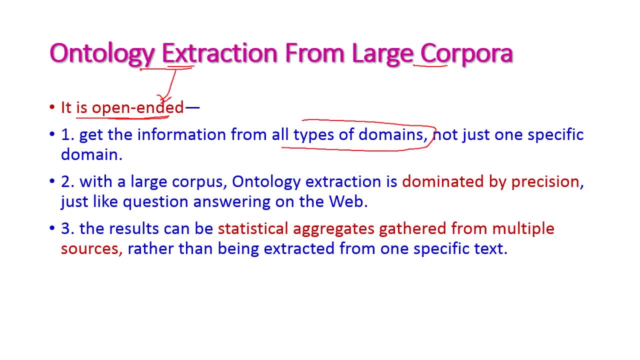 it gets information from all type of domains. ok, This ontology extraction is not dependent on k, It does not depend on particular specific domain, but it can accept information from all type of domain. With this large domains, that is huge volume of text, this extract. 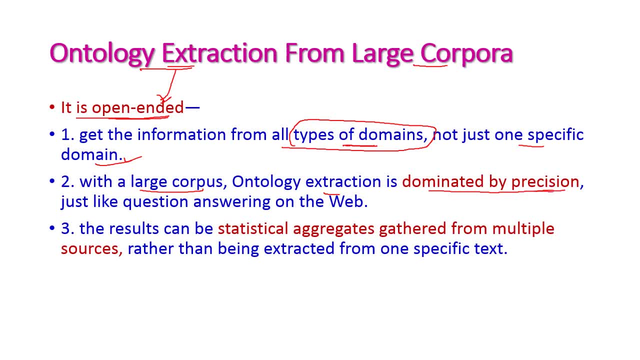 dominated by precision studies. the accuracy will be very high and exactly like question answering on the web, That means for a particular question it will give exact answer. Likewise the ontology extraction, The output will be very specific or very accurately, and the result, that is, the output, can be statistical. 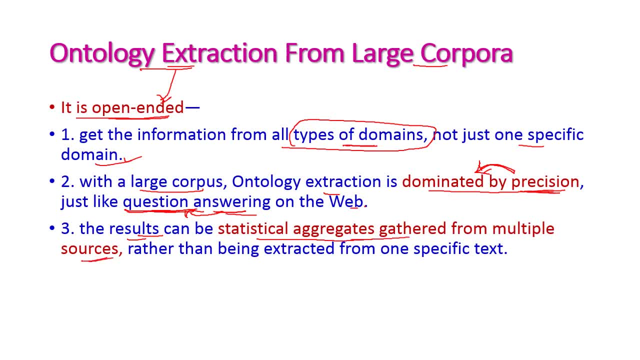 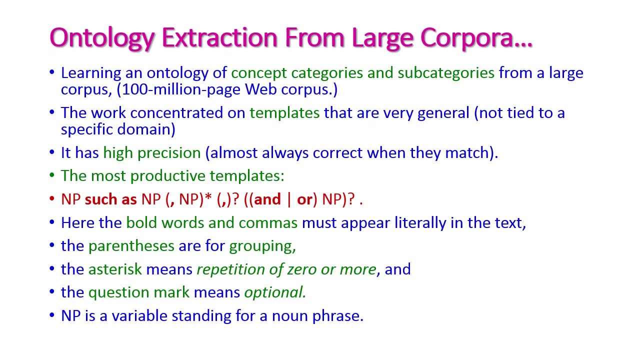 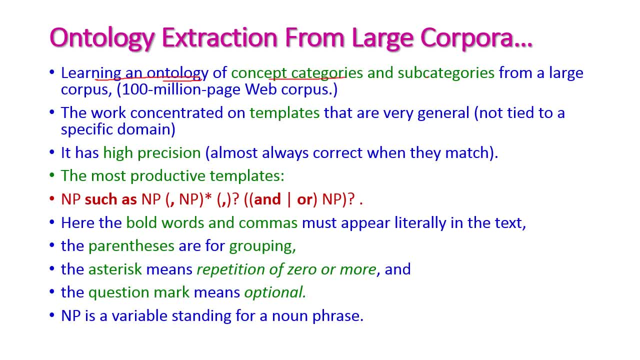 The ontology of Giant. that is what you see here by another method, in no one kháclining as the concept categories and sub categories from large corpus. OK, So the learning will be taken place by concept categories and the sub categories of concept from very large volume of text. OK, the text. 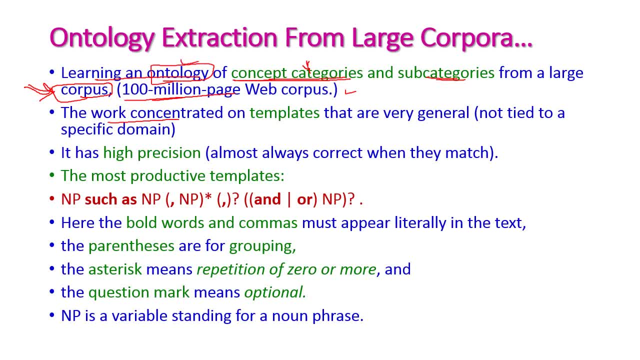 size may be hundred million pages. OK, This can be possible only in the ontology and the work concentrated on template, that is, generating template. There is one term which is nothing but summer: 그 י. cruelty, Beareful Life. when the subject gets vegetables and the substitute gets more trees and vegetables, the content gets 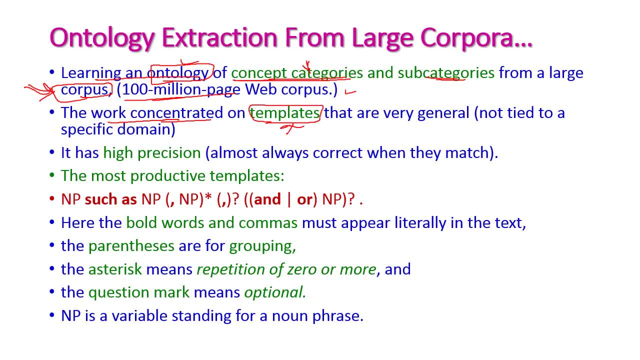 lower Gratitude For CPU usage. okay, So learning and ontology excels in Laurie Goodman minimum standard я. This is the Achield par templates and the template should be very general and this suitable for almost all the domains, not for a particular specific domain. ok, and it has high precision. that is the always. 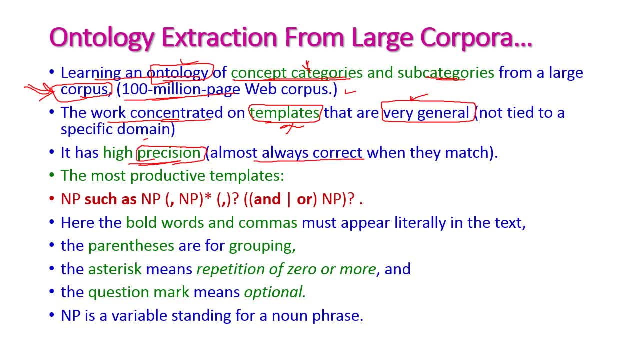 this should be always correct. that means almost always correct when they match. ok, if the concept will be map, then the template will be always suitable for everything and the most productive template. this is the common template. this can be suitable for all the domains that is noun phrase, such as noun phrase open, parenthesis. comma NP- close. parenthesis star- open, comma, close. 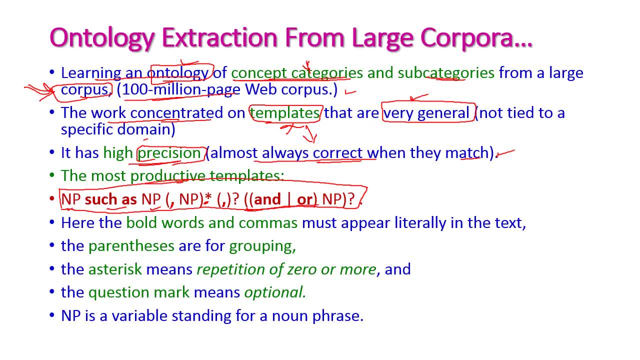 question mark and within bracket and or NP question mark. here the bold words and commas. the bold words and commas must appear in the text itself, ok. and the parenthesis- the parenthesis are used to grouping the text- and asterisks. this one asterisks means the repetition of zero or more number of times the same character and the question mark. 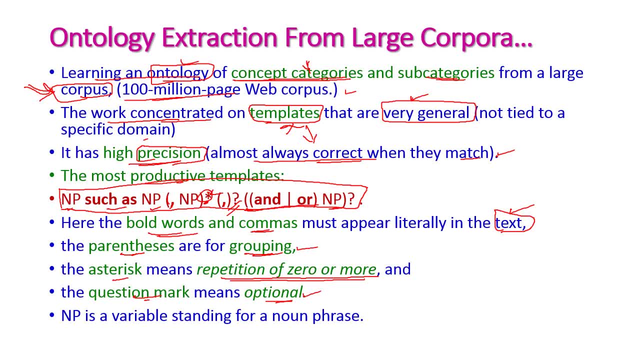 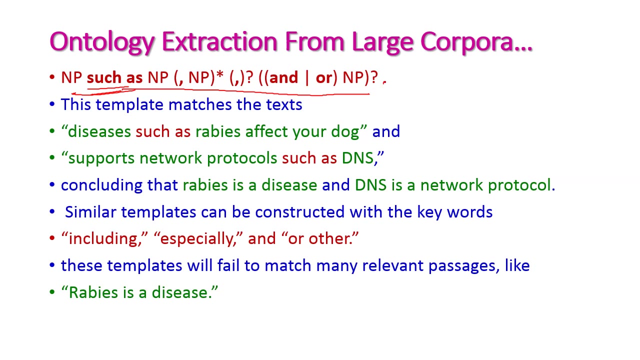 question mark means optional: ok, this may be present or not present. and the noun phrase: ok. NP means noun phrase, is a variable standing for noun phrase, and this is a variable standing for noun phrase. NP means noun phrase. this template can be matches any domain text. ok, that means a disease such as. 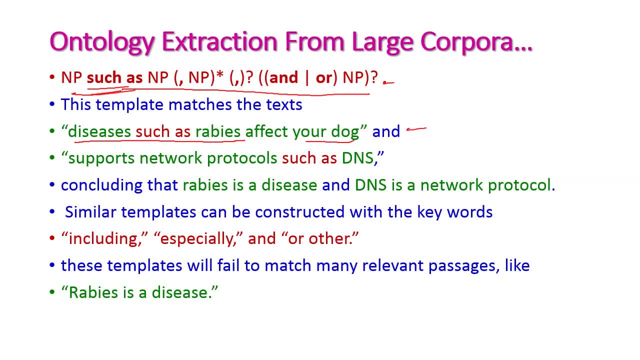 Robby's affects your top: okay. such as is a keyword which can used in this sentence and another sentence supports network protocol such as DNS. ok, so here we are using such as by using such as: see: so as is that keyword which can use used here, okay, and or are optional here: right, 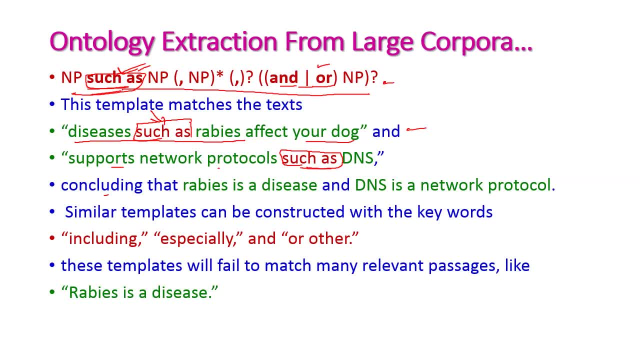 so the first text concludes rubbish is a disease and second one concludes DNS is a network protocol. okay, so the similar templates can be constructed with the keywords including: especially, and or other. okay, by using these keywords also, we can construct more number of term such sentences. here is another template. 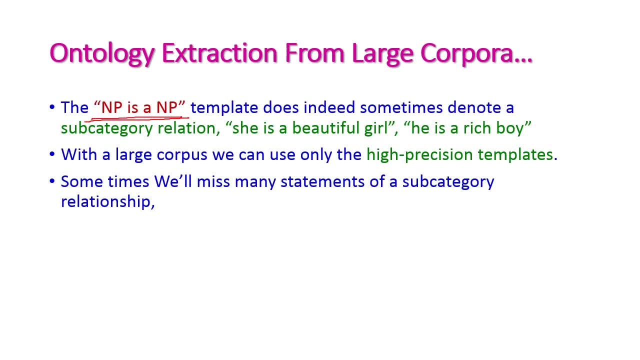 noun phrase: insurance is theczenia NP. okay, here is. here is the keyword. okay, by using this we can generate: she is a beautiful girl, he is a rich boy. okay, sometimes it is a subcategory relation. it denotes only the sub categories of the tutorials. okay, and another thing is: 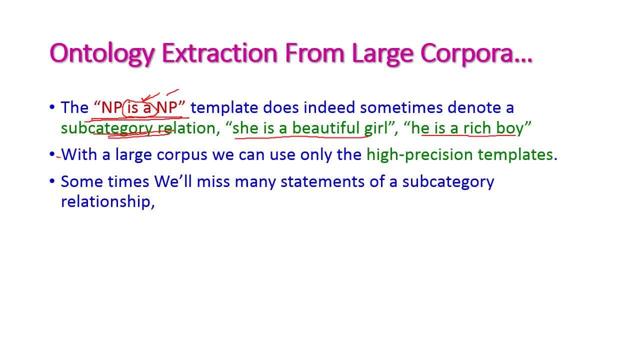 let us pity, words in a mouthного 222 can 주는 belief. professionals here relation And with large corpus, we can use only a high precision template. That high precision template means which we have used in the previous slide. okay, And sometimes we will miss many. 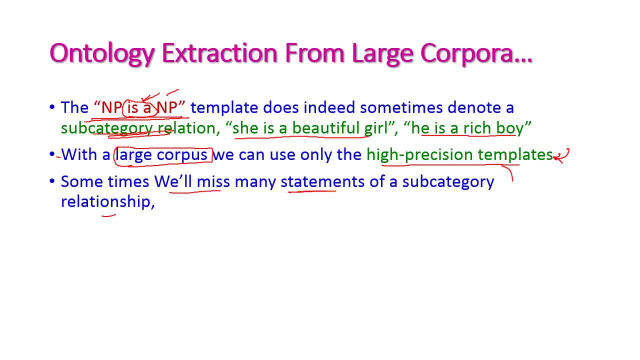 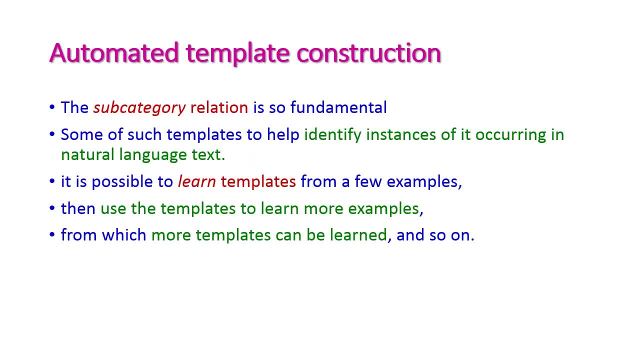 statements of subcategory relations. Suppose, if we use this high precision template, we can miss some subcategory relationship. Automated template constructions, that is, the template will be constructed automatically. right, The subcategory relation is very fundamental one, And to learn, 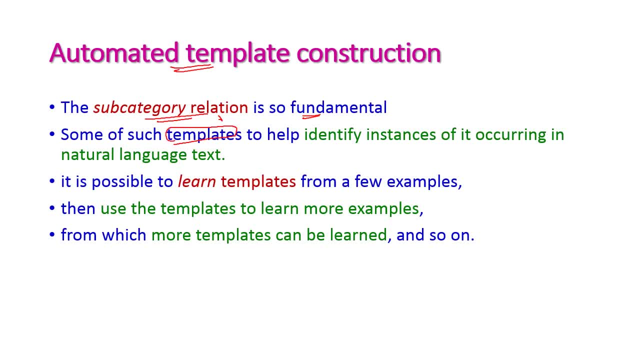 this. some of the template will be very much helpful to identify the instance of occurrence in the natural language text right, And it is possible to learn template from few examples. Suppose, if we give few example from this example, the system will learn the. 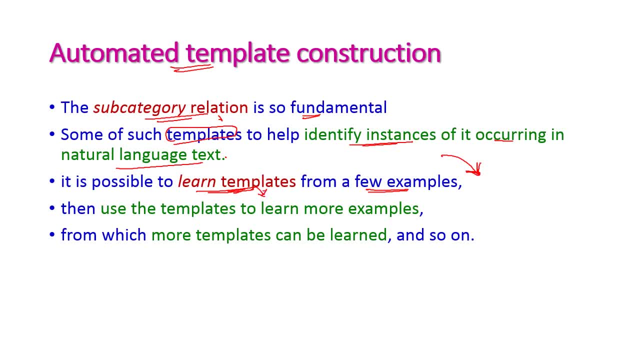 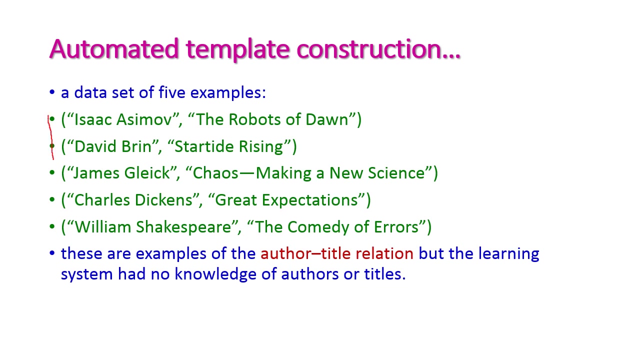 template And by using this template, the system will generate more such examples. From those example, it will again learn the template. okay, So likewise, the system will automatically generate the template. Here we are having five examples. So if we observe these five examples, we can easily understand that this is author-title relation. 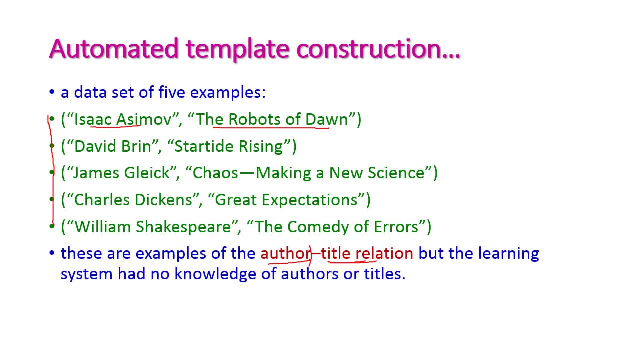 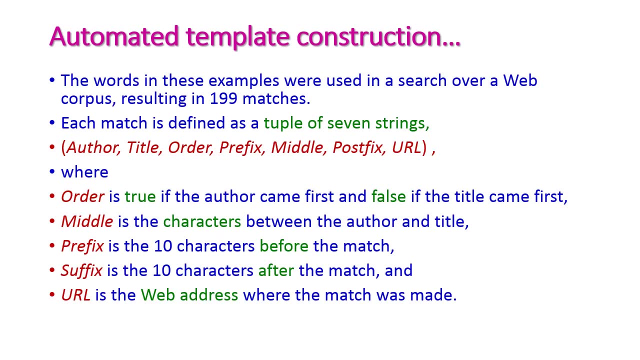 author and title of the book. okay, author and title of the book relation, But when come to learning the system, the system does not know any knowledge about the author or titles. The above given words are used to search on the internet, And this is the system that is used to search on the internet. 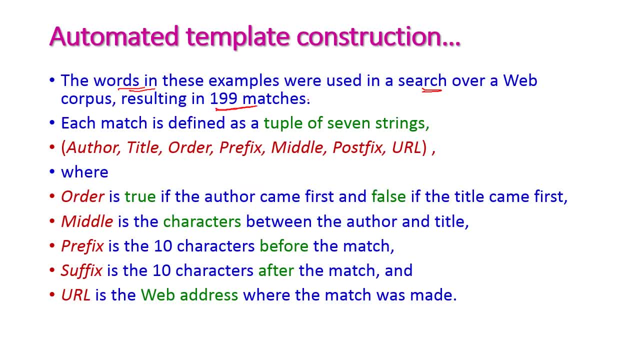 So, which is the first example, Here we have a table. So we have a table. This will give 199 matches and each match will give the tuple of seven strings. The seven strings are: author, title, order prefix, middle a postfix and urn. Here order order is nothing but which. 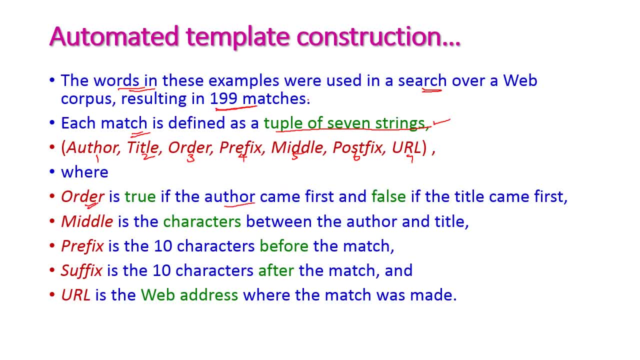 will come first. If order is true means author will come first. If order is false means the title will come first. Okay, this is a command. Well, there are two commands here. There are two test, there are two settings. There is a test called test. That is where 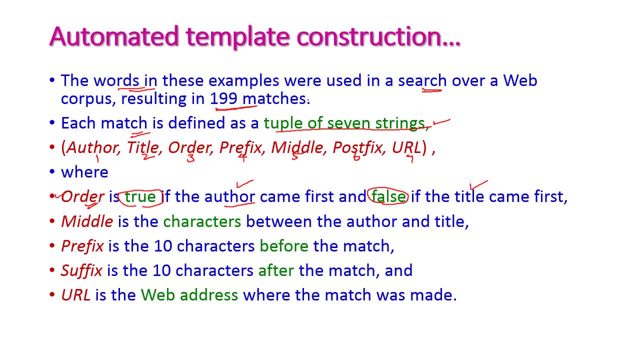 you get the test. A test of test means that you have to identify text. I will show you. This is called as order And second one is middle. Middle is nothing but the characters between author and title. Okay, That is called as middle, And prefix Prefix means the 10 characters before the match. That is prefix Suffix means 10 characters after the match And URL is nothing but the web address where the match was made. Okay, 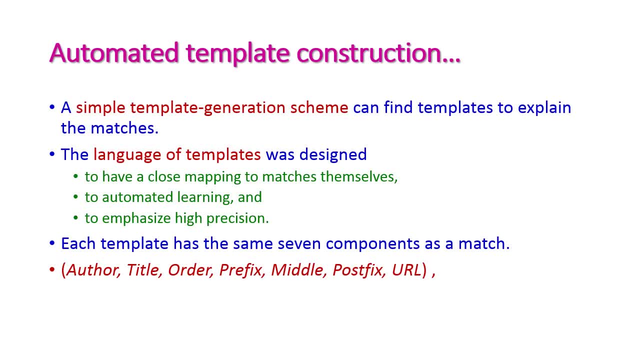 Okay, The simple template generation scheme which can find the templates to explain the matches. Okay, Here the language of templates that is designed to have a close mapping, to match themselves and to automated learning and to emphasize high precision. Okay, And here the each template has same 7 components. 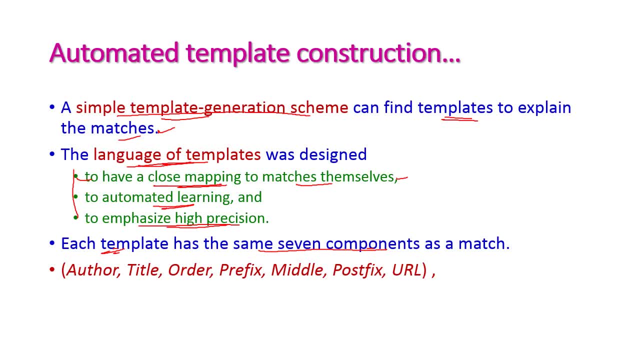 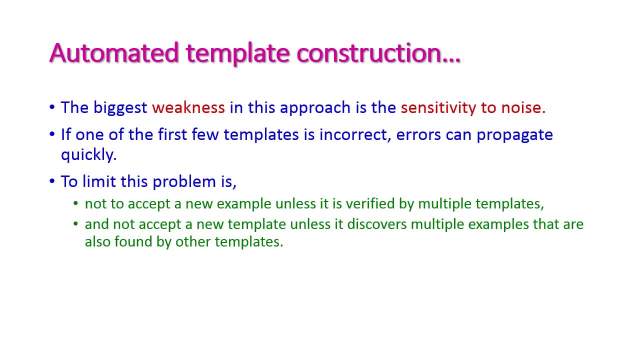 That matches The 7 components we have already seen: Author, title, order, prefix, middle postfix and URL. The very big drawback of this particular approach is sensitivity to noise. Okay, If there is any noise, then there is a problem to generate the template automatically. 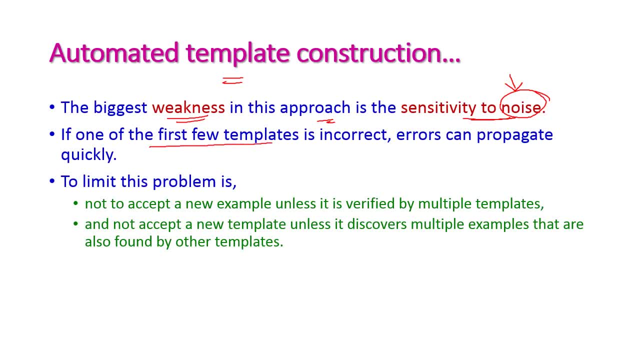 That is, if the first few template is incorrect, The first few template is incorrect, Then error can propagate quickly. Okay, To overcome this problem, First one: Not to accept new examples unless this example will be verified by multiple times. This is the first approach. 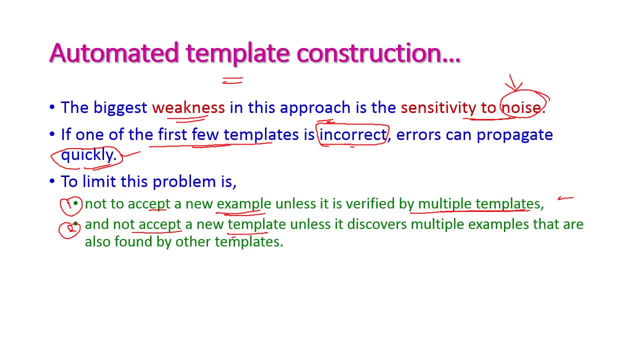 And second one: Not accept the new template unless it discovers multiple examples. So the template should discover multiple examples, Then only it will be accepted. And thirdly, there is a kind of softwareитесьless to start. But if this template is not found, or if it is not realized, then what to do? 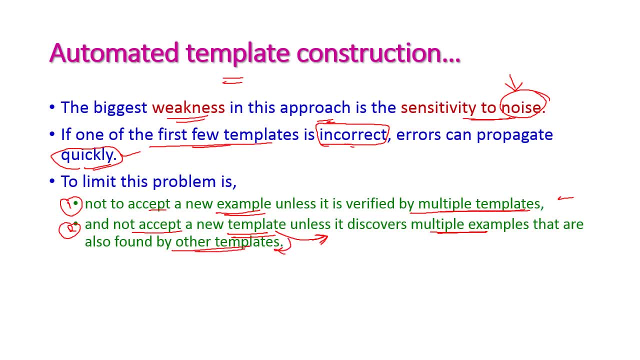 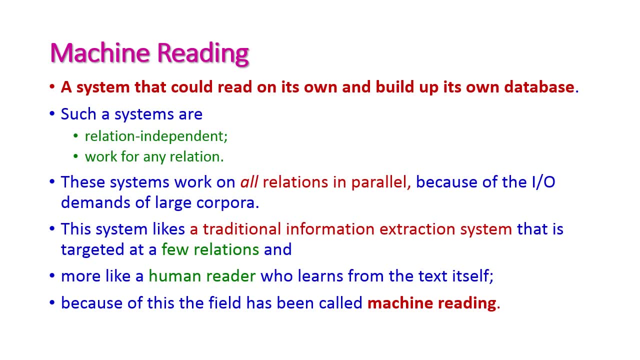 The какое proof editor tool is the most potent category. This nosso service title. you can see in the screen. It shows various templates, And this is also found by other templates. Okay, So by using these two approaches, we can easily overcome this weakness. 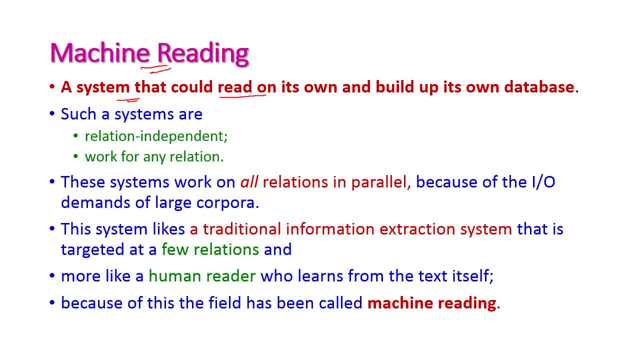 Machine reading. Machine reading means a system that can read by its own and it can build its own database. Okay, This is called as machine reading And these systems are relation independent systems, That is, it can work either on remote or it can work by system management. 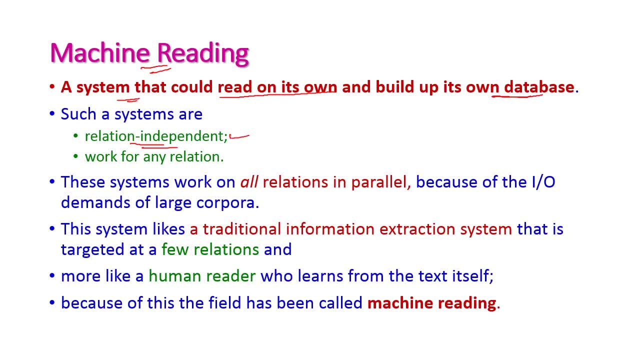 And this is actually a topic. That's why what you just seen, Okay, What is the commence 꿈 command on computer? What are these methods to understand? and They work with machine reading on any relation. okay, there is no dependent on the relationship and this system can work on all. 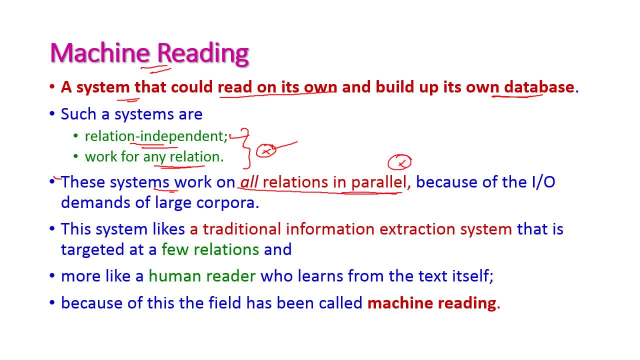 relations in parallel. this is important because the I vote demand of very large corpora right and the system likes traditional information extraction system that is targeted a few relations and more like a human reader, how we are reading. by reading the text, we can learn something, isn't it? likewise, the system also read and it can understand something from the text. 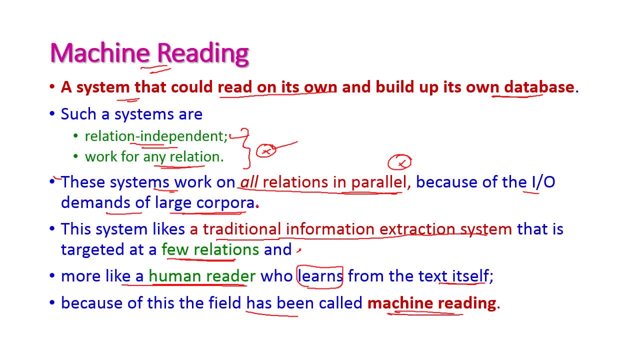 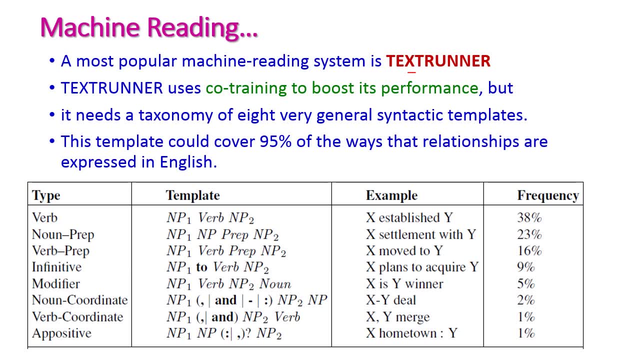 hence this field is called as machine reading. the most popular machine reading system is text runner. this text runner uses co-training to boost its performance. okay, but this needs some taxonomy of its very general synthetic templates. okay, it synthetic templates are given here in this example and this template could cover 95% of ways that relationship are expressed in English, right? 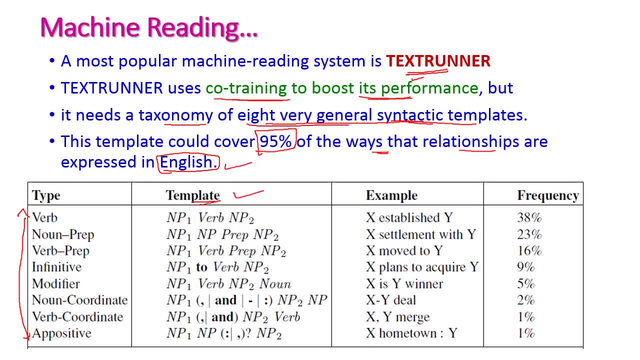 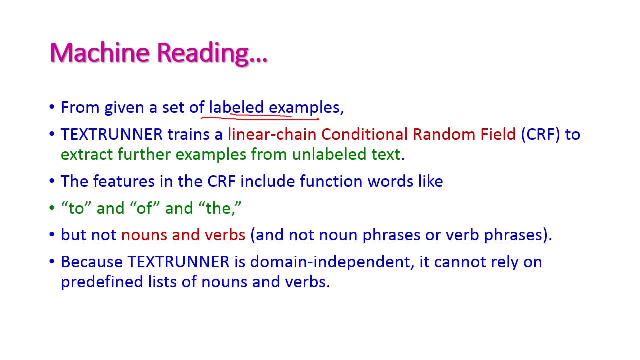 so the template. however, if you are using, you are looking to explain that context. so this line: Bush, what? what do depth like two of the? okay, and it never include nouns and verbs. okay, because the text runner is domain independent, so it cannot rely on the predefined list of nouns and verbs, right? 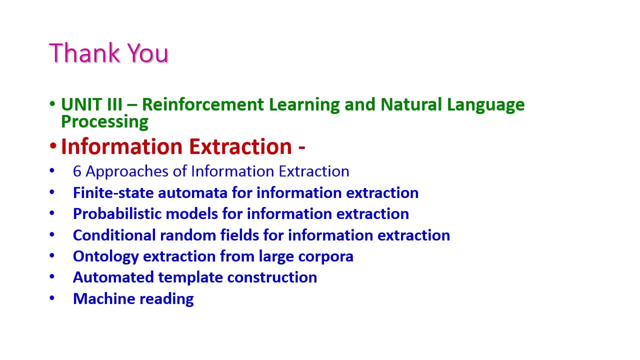 so far we have seen the information extraction, that is, ie from third unit, that is, natural language processing, and we have seen six approaches of information extraction. the first one is finite state, automata, probabilistic model and conditional random field for information extraction, ontology, extraction from large corpora, automated template construction and